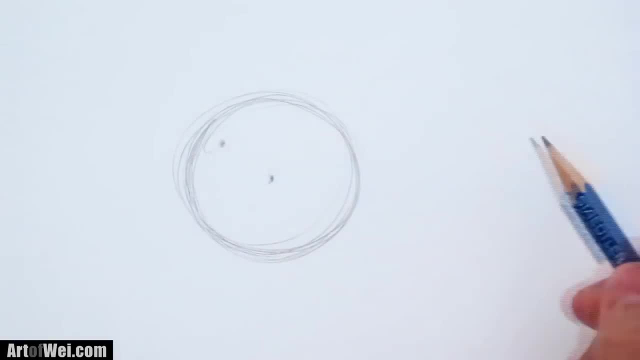 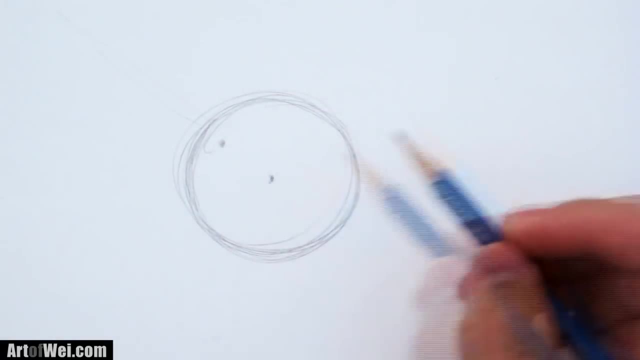 anywhere in the sphere. Just pick the hottest spot. Let's say that's going to be the highlight area. So the light is coming from somewhere. from here, This side, This is going to be the brightest part. So a quick way to do it is just to from the center point to the highlight. 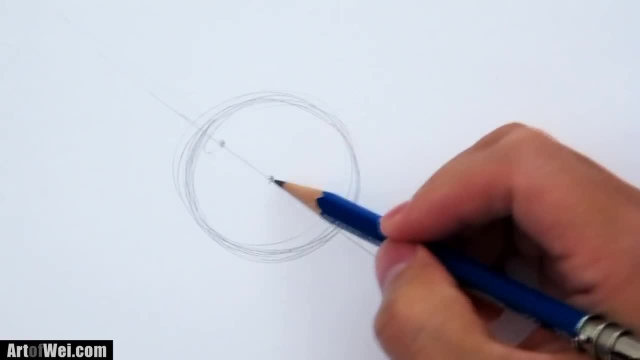 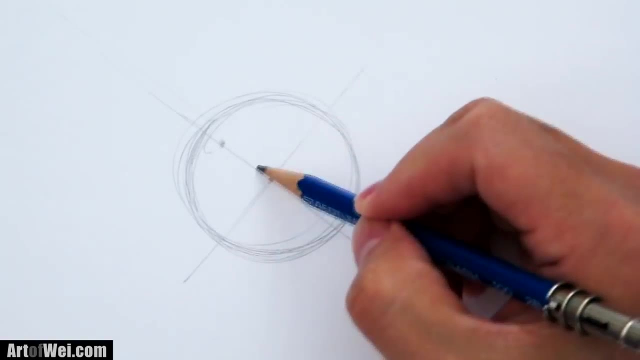 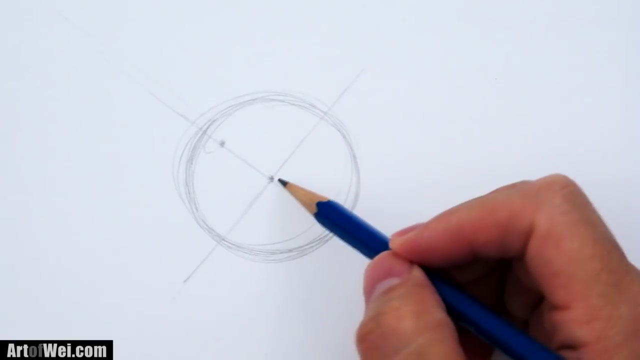 draw a line all the way across And then, from the center, draw a line that is perpendicular to this line. So you're just going to basically make an X, Because this is going to be 90 degrees. So once you have that, now to figure out where the shadow will end, where the terminator. 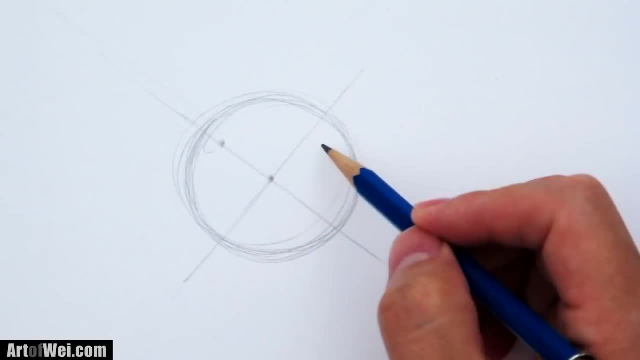 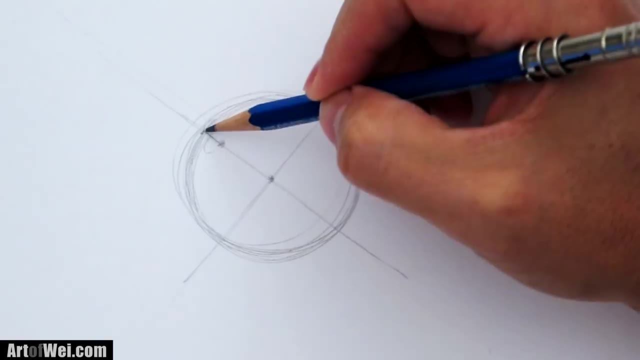 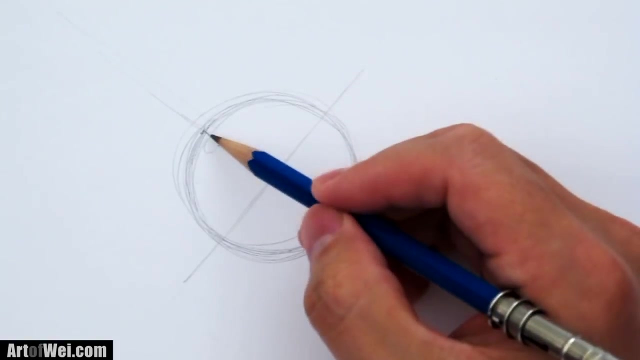 is where the light will not be hitting the surface of the sphere. Just calculate this distance right here to this distance. So you take this distance right here and you duplicate it here, So it's going to be right around here. So the distance from the edge to the 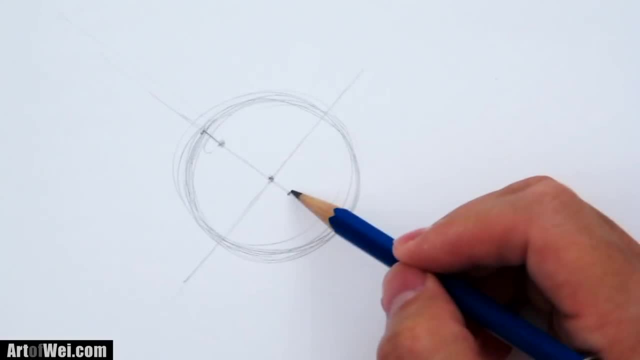 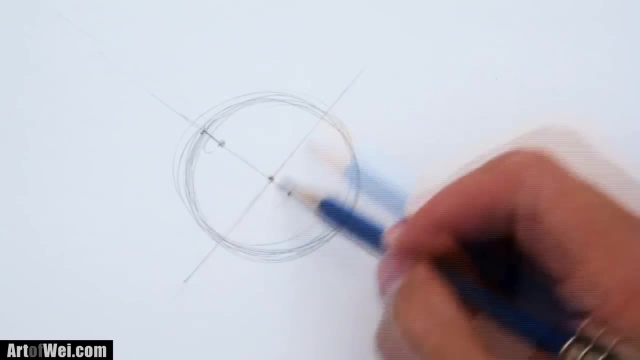 highlight From the center to here. So once you have this now, you know the terminator is going to be right around here. So what you need to do from here is to draw a kind of like an ellipse, As if you're slicing this. 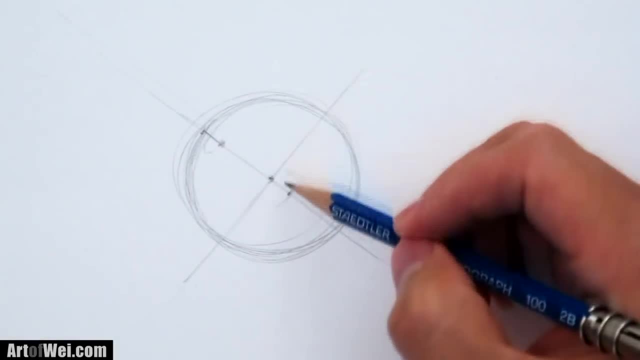 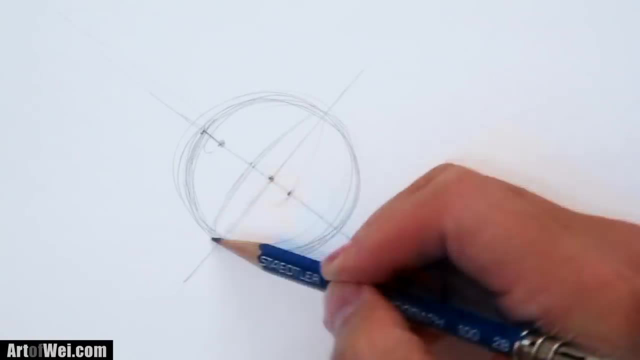 sphere, you know, through the center at this point. So the ellipse. obviously you can double this area right here. This is going to give you the ellipse shape. Now, this is the part where it gets a little bit tricky, because you're going to have to be able to draw an. 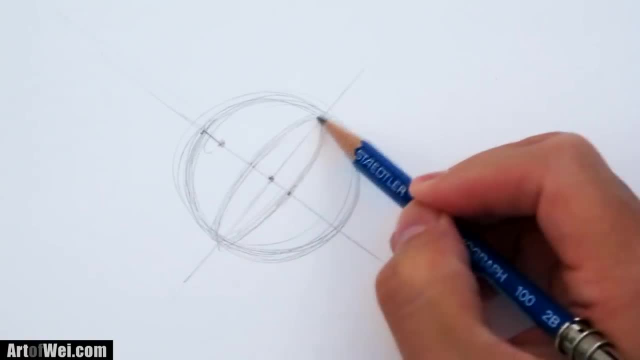 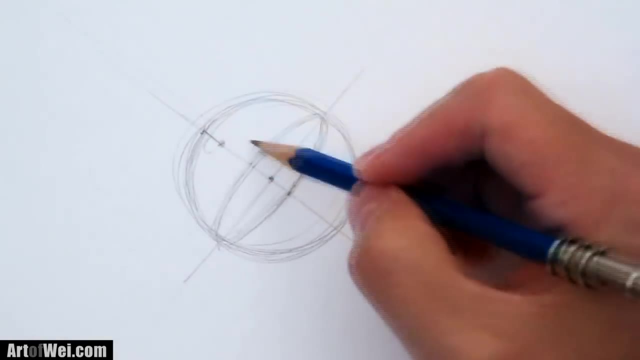 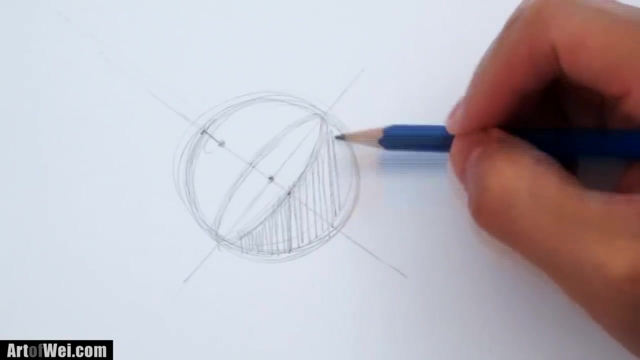 ellipse. Okay, And I'll talk about that as we go on. So now that we have this ellipse right here, now we know that the light is going to die off right around here, So everything behind here is not affected by the main light source. 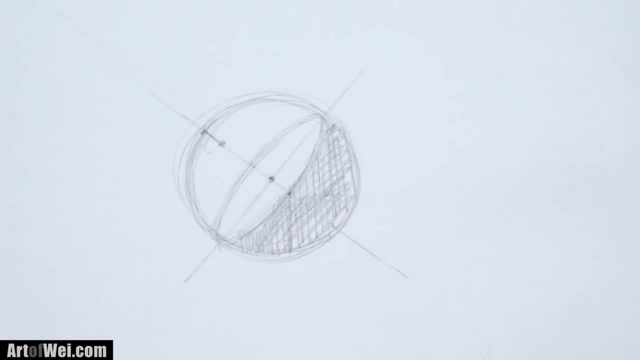 So this would actually be like: let me switch to a 4B. I was using a 2B pencil, So this would actually be like the moon, right? So if you were to draw the moon and trying to figure out, you know how to. 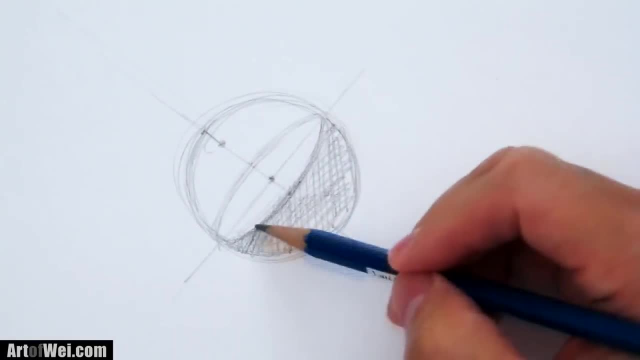 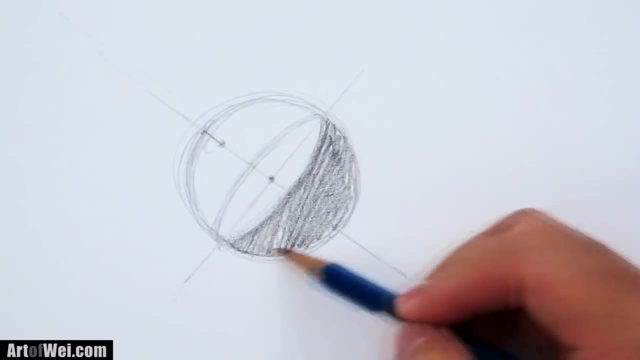 shade it, you figure out where the light source is, where the sun is, and then you can, you can calculate it like that, And then this would be your moon And pretty much this whole area would be completely dark, because there's there's really no light reflecting back onto. 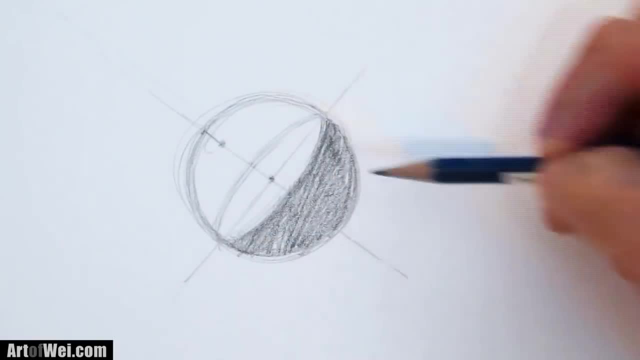 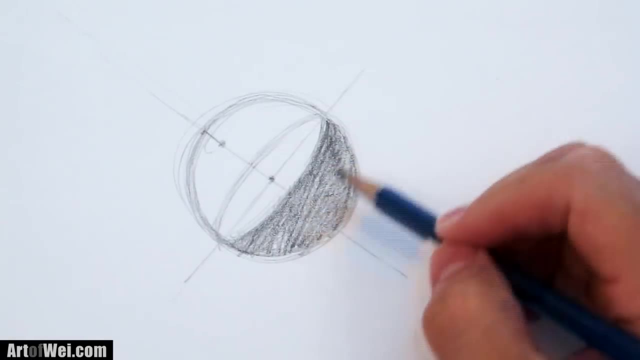 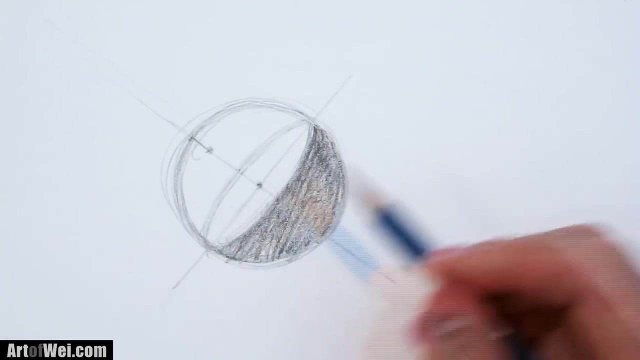 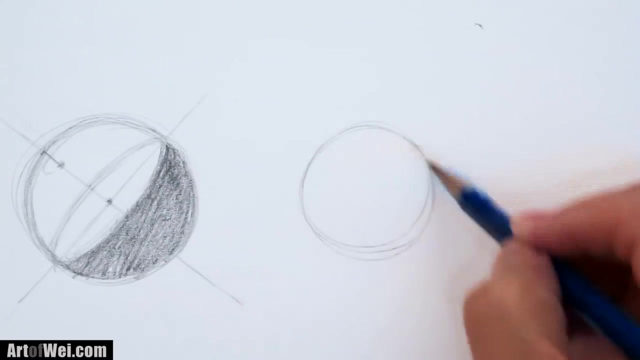 the onto the moon. Okay, So now, obviously, if you're going to shade a regular sphere, it's not going to look like this just because it's a different light source, right, But we have to understand how this works. So, basically, how you would shade a moon, let's just do another one real quick And then once. 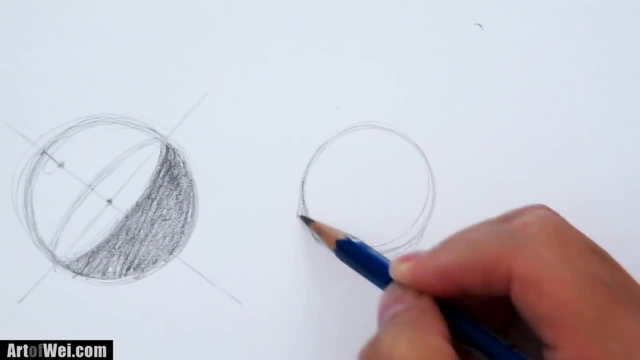 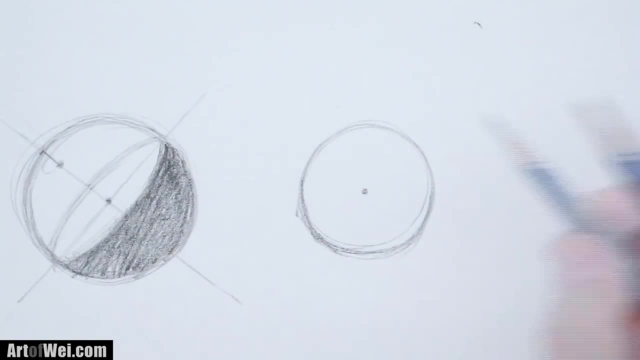 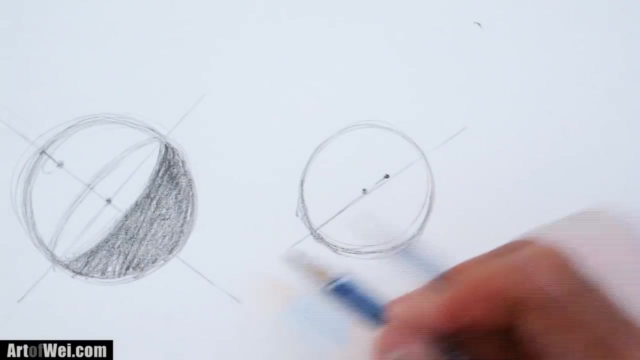 we understand that, then I'll move on to how you can actually shade it. You know that's a real sphere, not necessarily just the moon. Okay So the center. let's just pick any light source Right around here. Okay, So this is the brightest area right here. So I'm going to draw a line. 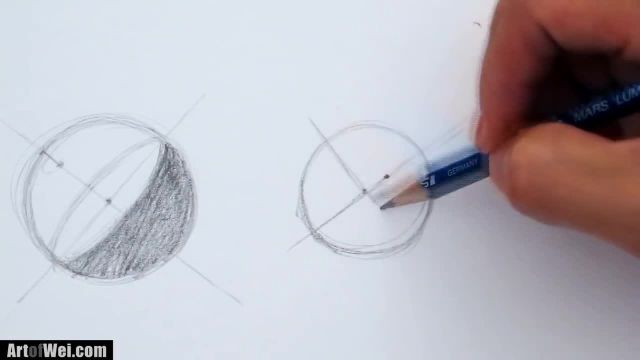 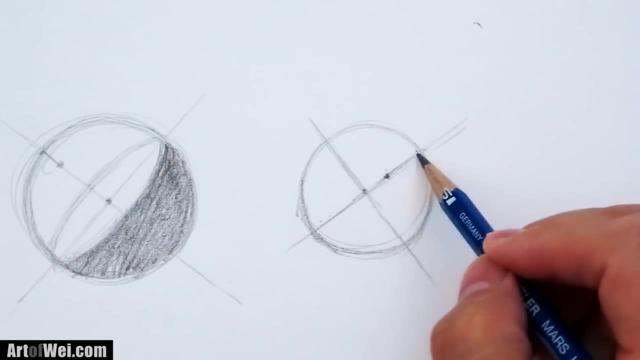 Okay, Line straight through and then a perpendicular line to the middle. Okay, Now take this distance right here, push it over here. this distance, push it from the center here So roughly, probably right around there. So now you have the center and this is where the light's going to end. 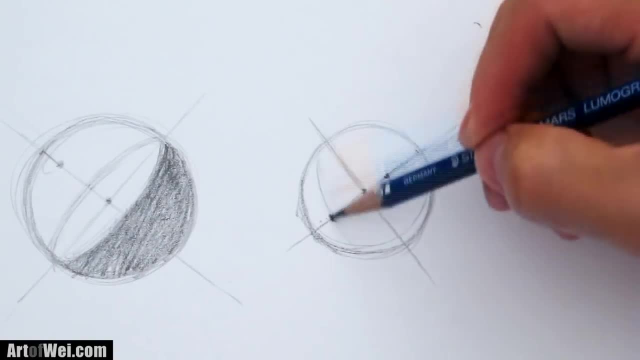 So we're going to draw an ellipse right here inside, all the way through. Now the real reason I'm drawing all the way through, even though this is everything's behind, let's just say I'll put in a dotted line. It's just that way you can see it, and it's actually. 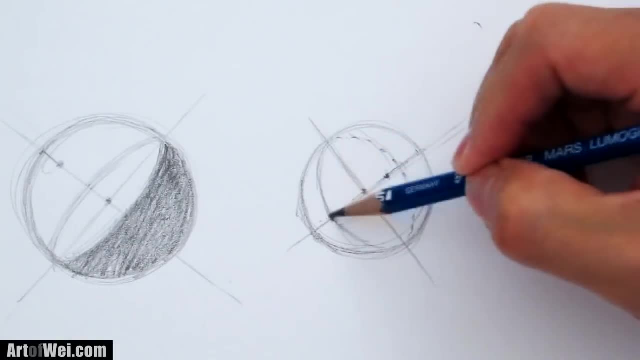 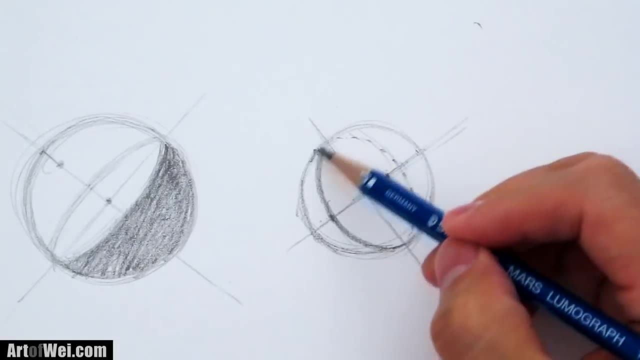 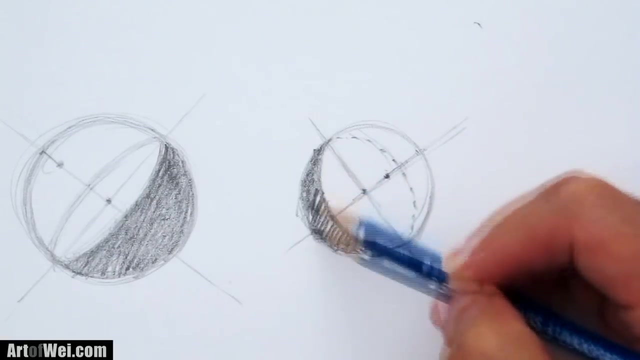 it will assist you in drawing this curve, Okay, So, so, let's do this same thing again. We're drawing the moon again. Okay, So, with this method, you can actually see the moon. Okay, Okay, Okay, Okay. 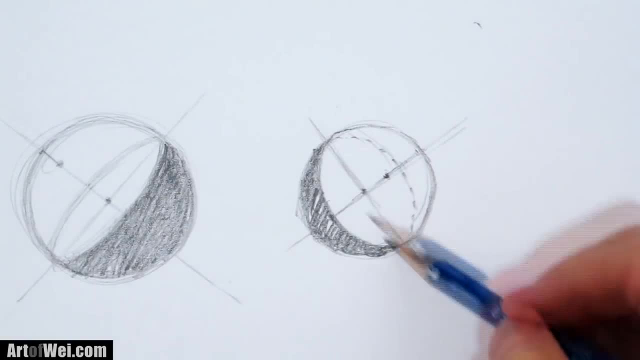 Okay, All you have to do is actually pull it in a bit more, this angle. So then, with the dilemma that you're basically essentially doing the over Titan, now you can, you know, quickly get a sense. you know where this nail, the, the light is going to be terminated, where 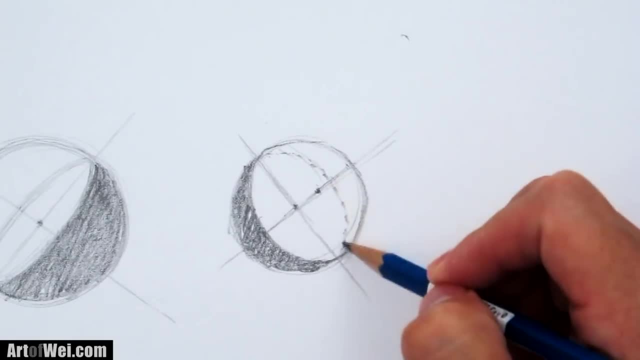 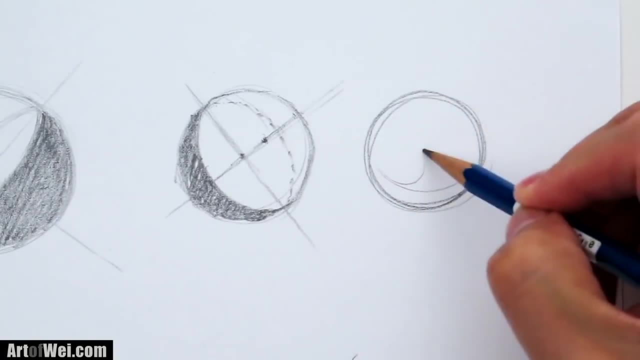 it's not going to hit the sphere anymore. Now, let's see. now, All right. So the reason why I like to draw the back of it too is because, if you are, let's just say, let's say you do, do this again. 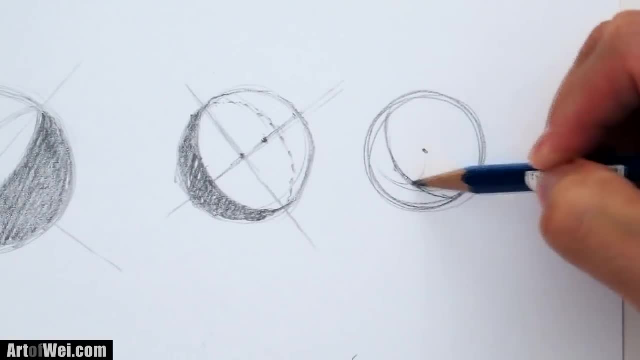 Okay, And I'm here and I'm trying to draw this. You know you, you might do something like this, and then you realize this is probably a little bit too sharp. as we do to the back, this right here is a little bit too sharp. it actually needs to round off more. so if so, if you draw the back, 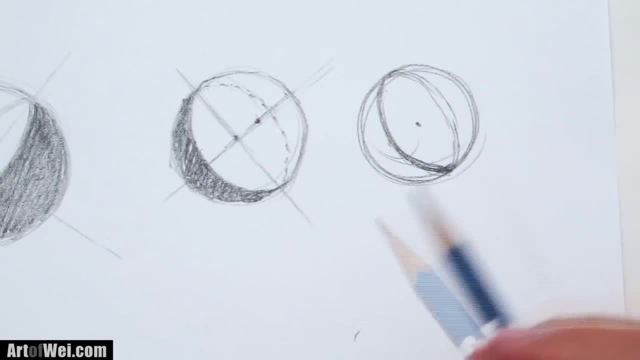 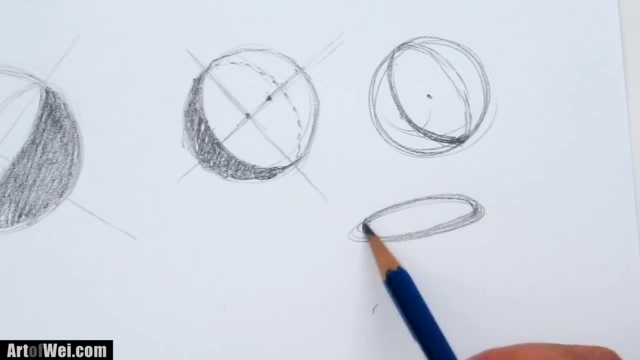 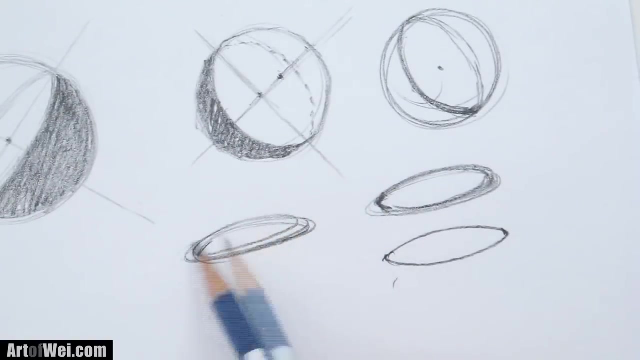 more. that way you can see the ellipses. it's nicely round. it's like if you're doing an ellipse, see, see, this would be more accurate, right, then if you do this, see, this is not accurate because this is too sharp right here. so that's one of the reason why you want to just draw the whole thing, at least at. 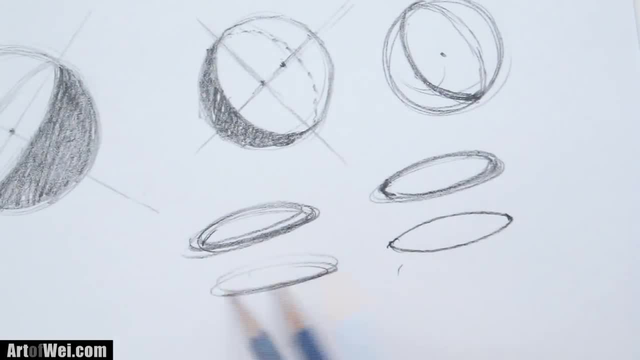 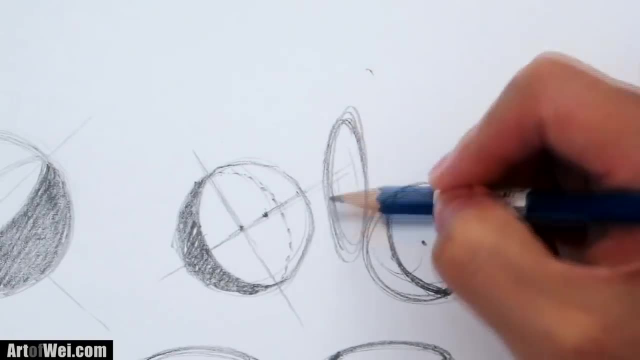 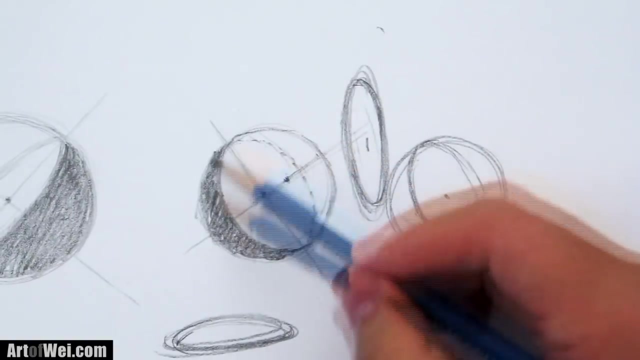 first get used to doing these kind of ellipses and it's difficult, you know. that's why they have templates for this kind of stuff, because if you need to draw something accurate, you know, like cars and stuff, you really need the ellipses. but you know this is just a very rough and dirty way. 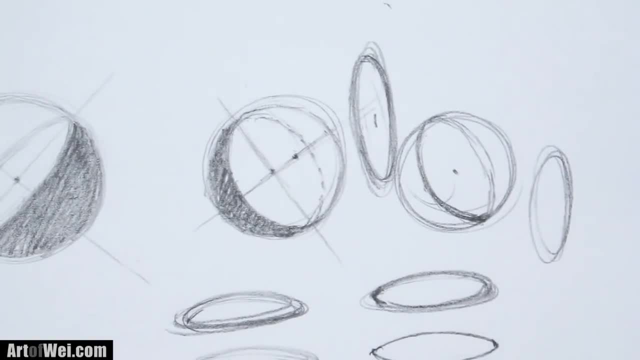 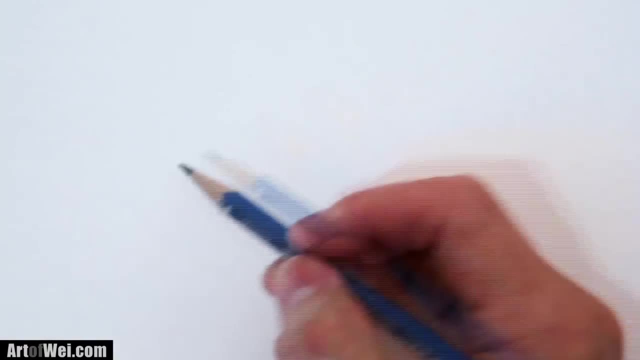 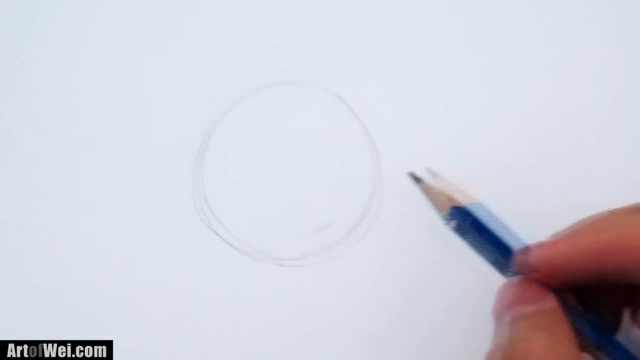 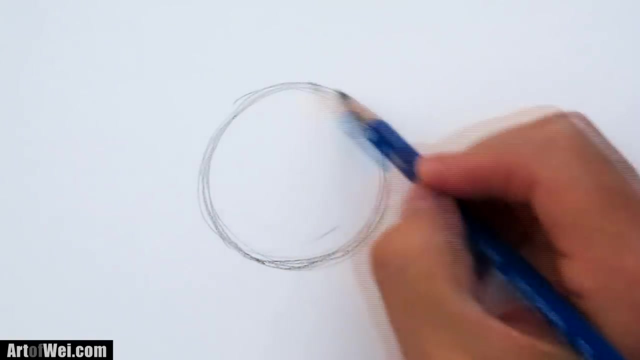 of drawing ellipses, but it's good enough of what we're trying to do here. so let's do a real, a real sphere and not just the moon. but it's just gonna be the same method, but we're gonna shade it a little bit better. okay, so let's start off with a sphere again: the circle. okay, so we're gonna find a. 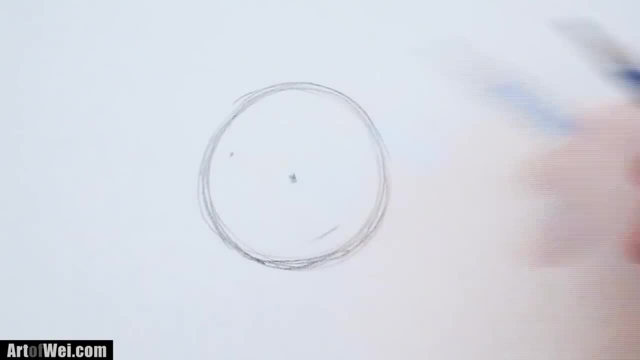 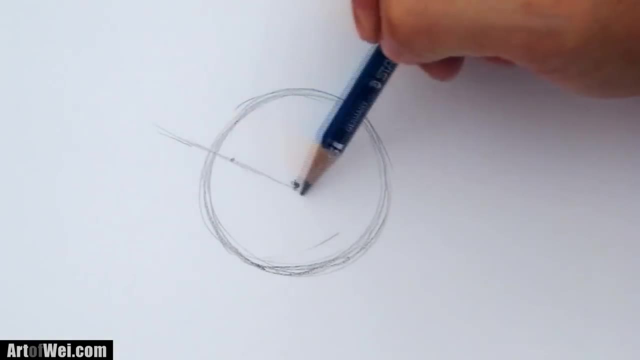 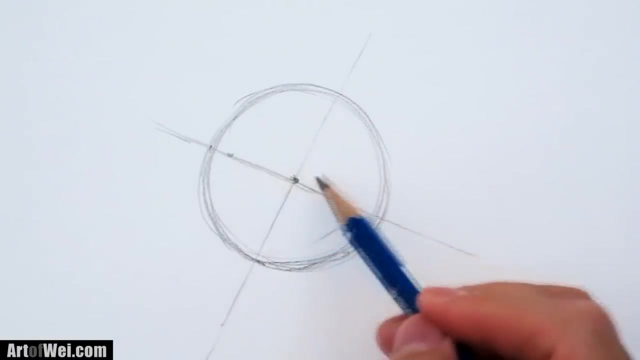 center, let's do the light, okay. let's just say somewhere right here, okay. so here's a center, the light source, hot spot right there. so I'm gonna draw a line and draw a perpendicular line from the middle. take this distance, double it over here. so it's gonna be. 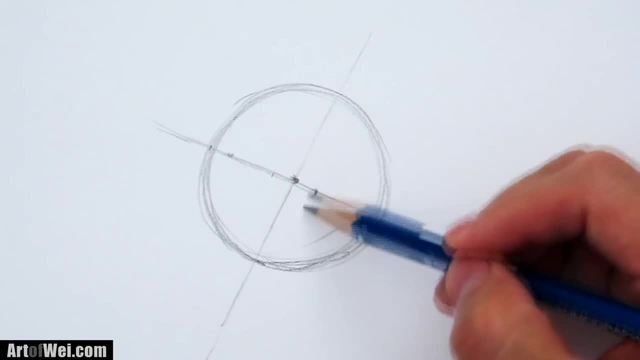 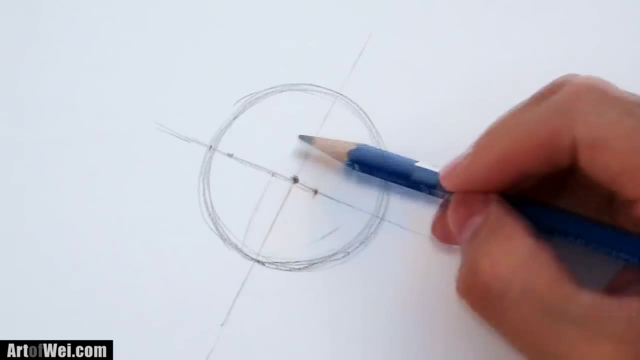 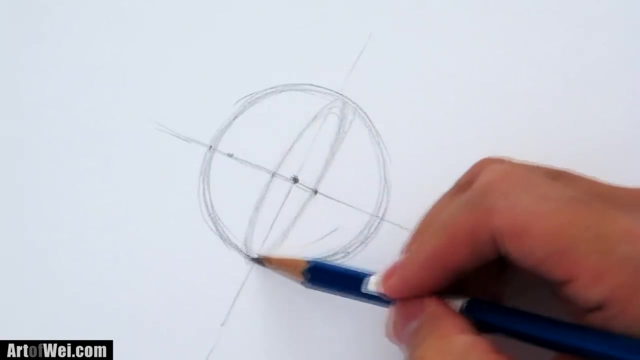 right around there. now we draw the ellipse. you can just, since this is the center. you know, this is kind of equal distance, so you can just put this distance over here. so now we're gonna draw the ellipse as best as you can. you know, I mean, even if you screw up the ellipse, it's as long as you get it. 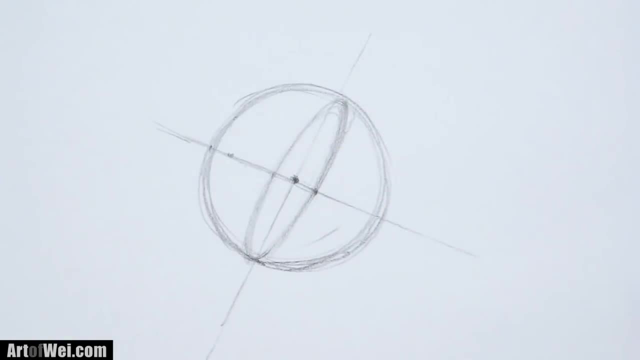 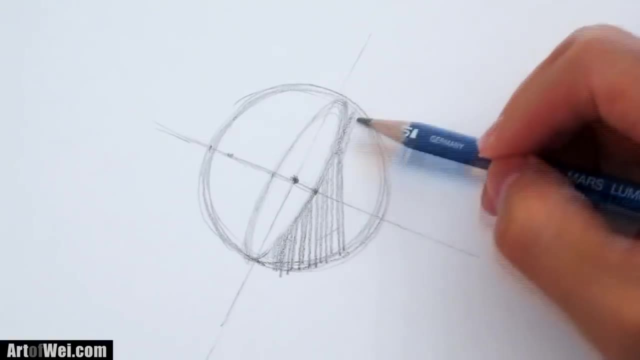 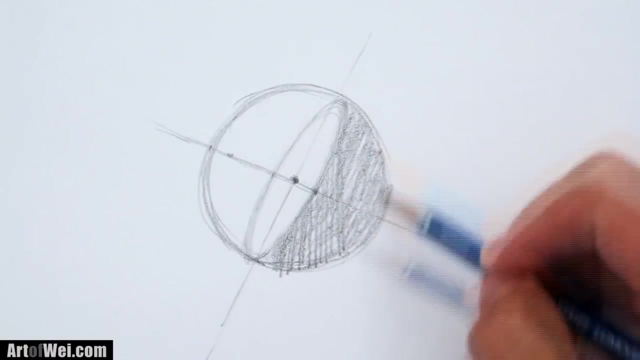 close because we're gonna- we're gonna- shade the heck out of it anyways. all right, so let's go. okay. so now we know this is gonna be not affected by the light source, so I'm just gonna give it a little bit shading and this will be affected entirely by pretty much the environment. okay, so now we know. 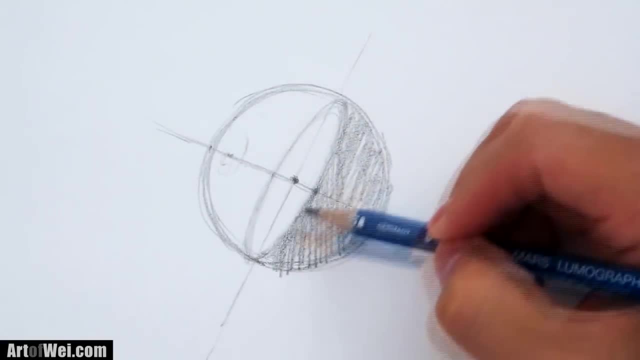 this is the hot spot. so we're gonna do a little bit of shading and then we're gonna do a little bit of shading and then we're just gonna delay myself with the suitable. doesn't matter how long we do it. you know I want it at this point of time something to really show up. I'm gonna show you. 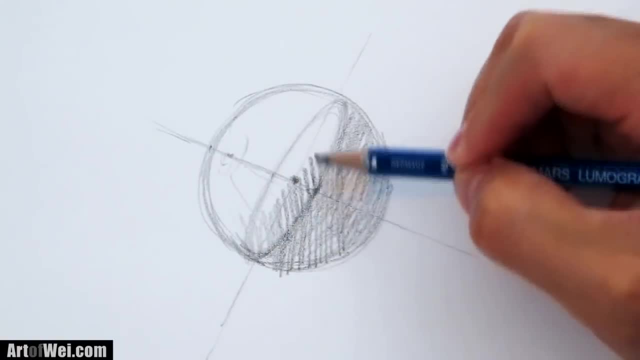 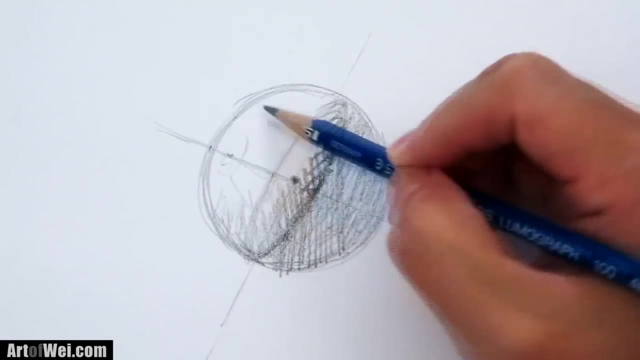 for now. okay, so let's go ahead and I'm just gonna come in and this is what this is. it's the Red Hat's in here. this is the Red Hat and this is the Lightist pot and this is gonna be the darkest part, so let's. so. everything from here is just as basic a gradation from dark to. 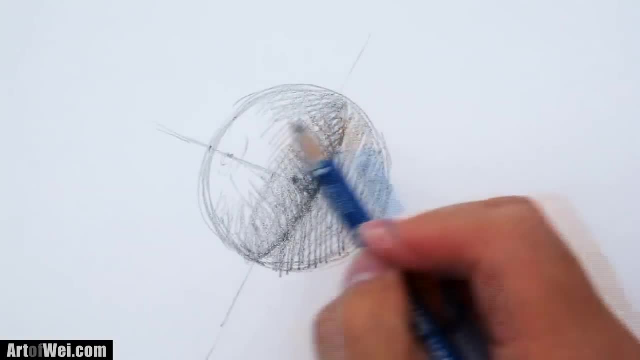 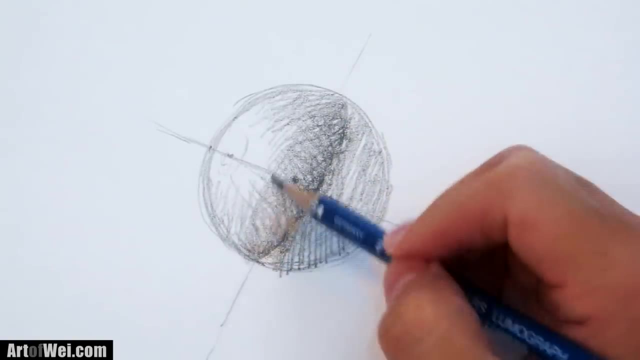 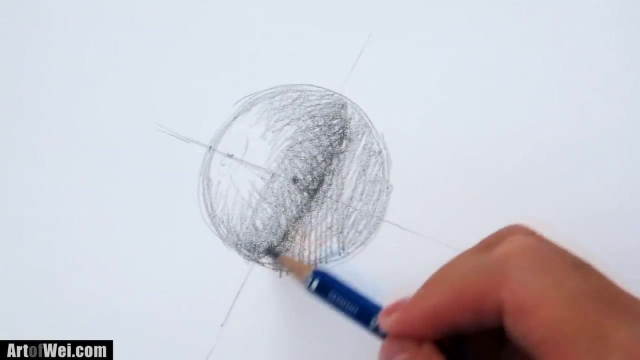 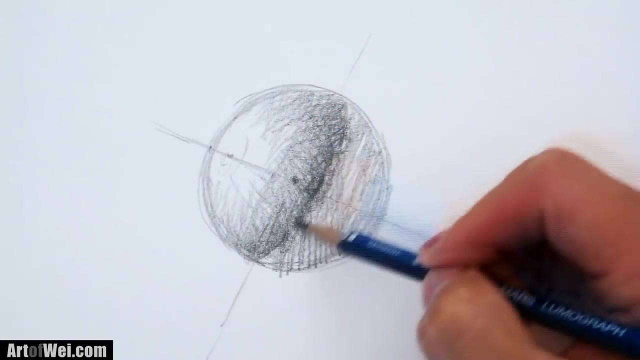 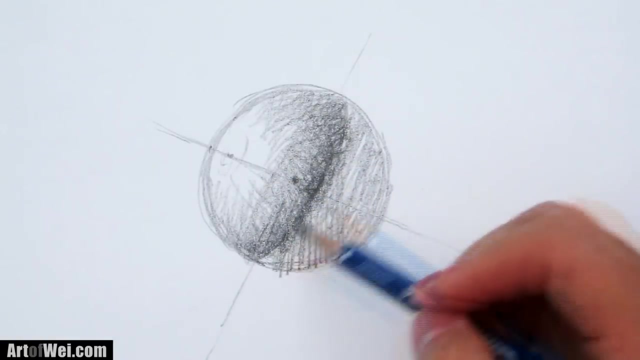 light. so I'm just gonna start off out here again. I'm using cuarto, Okay. so now you kind of see the shape forming a little bit. right Now you kind of feel that this is a sphere, not a circle. So obviously it all depends on light source. 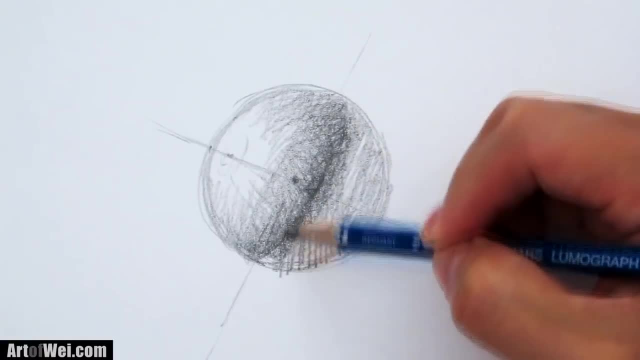 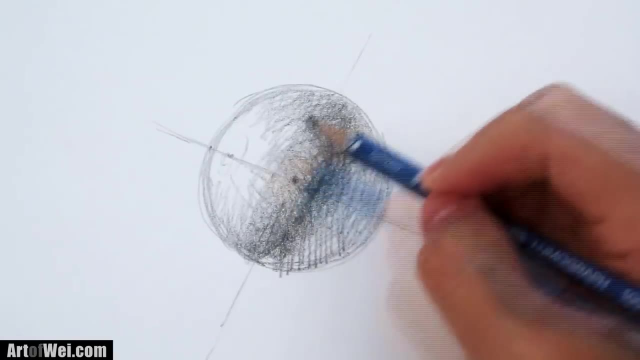 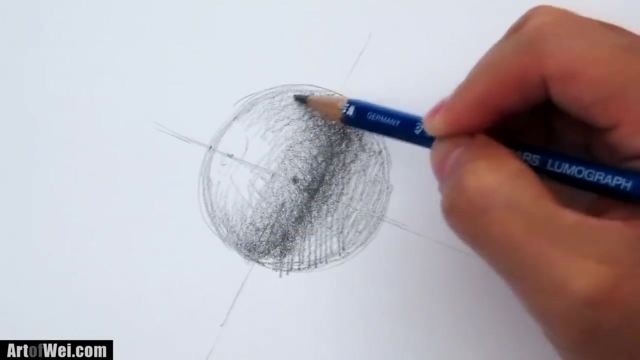 So you might want to soften that up a little bit. So I'm just going to soften it up. The light source is a very broad light, you know, kind of like soft lighting, not a point light. A point light would be like the sun. 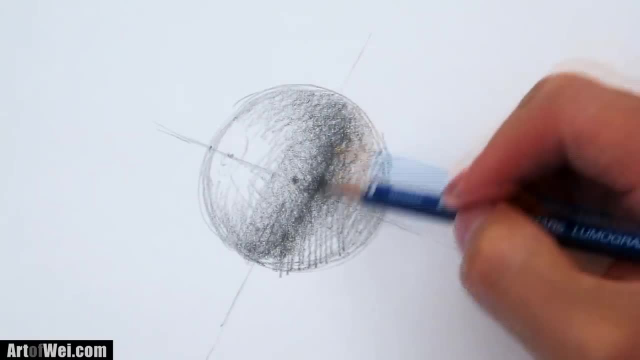 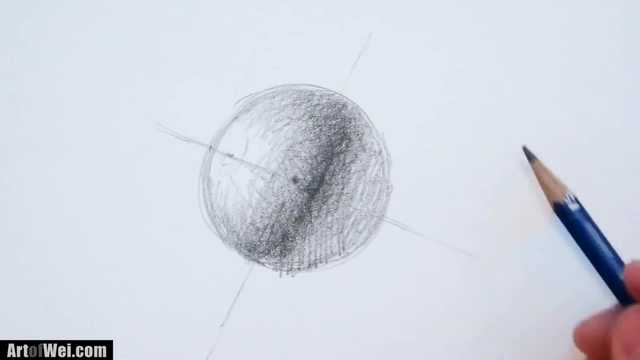 That would be like the point light, because it's really bright and it's far away. So now you can kind of smooth things out. So now you can feel it a little bit more. right, Let's just put this on the table. Let's just put this on the table. 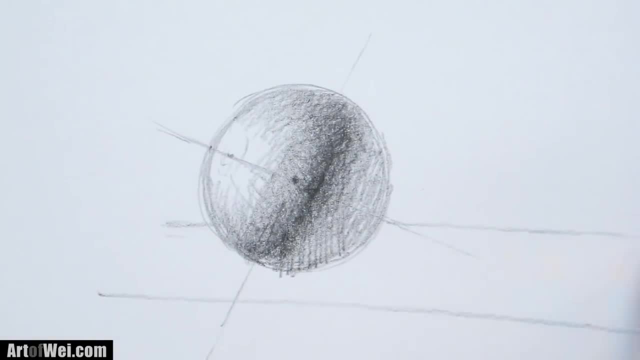 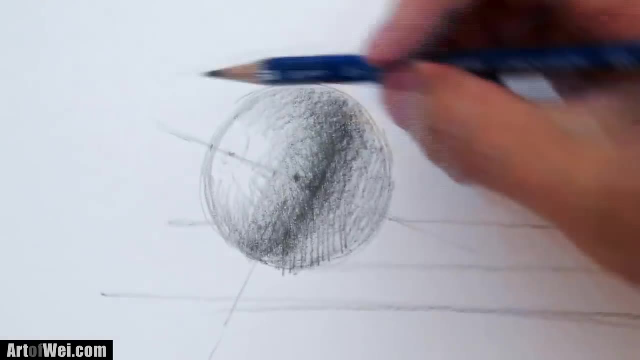 Let's just say this: way we can visualize this thing a little bit better. All right, so I'm not going to go into detail, too much detail into this. The light direction is here so we can go right there. So the shadow is going to end right around here, right? 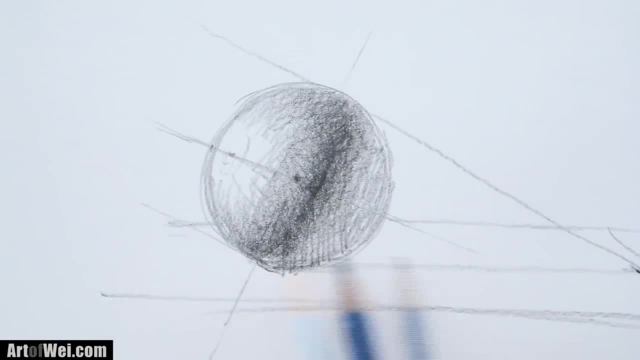 That's the top, And the bottom is going to be right around here, right? So the bottom, this whole area, would be like basically an ellipse, right? because that's what it is. It's just a circle. It's a circle with a shadow. 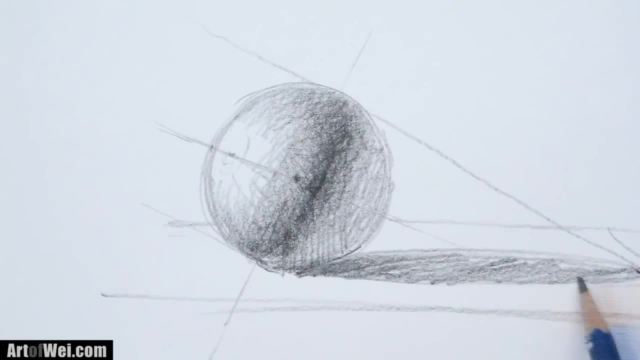 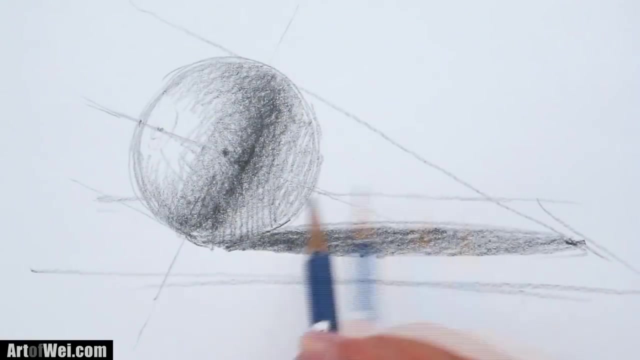 So this is going to be dark and this whole thing will be dark, And the only light this thing would get is basically the shadow. we get is anything from the environment. All right, so let's do that. And then now you know, now that you put in this, this seems a little bit too light, right? 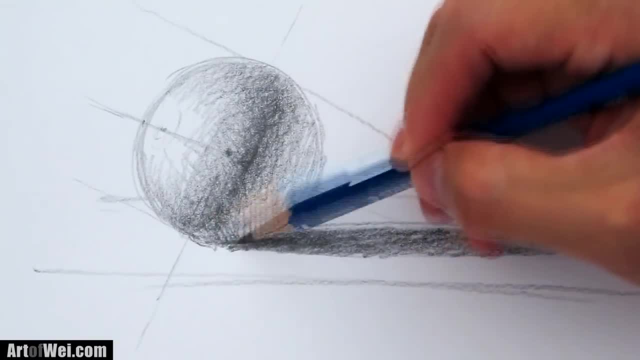 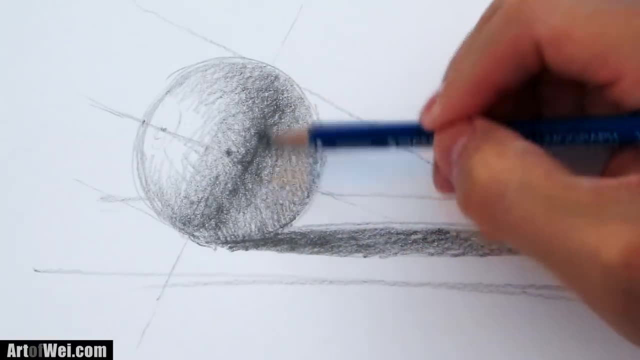 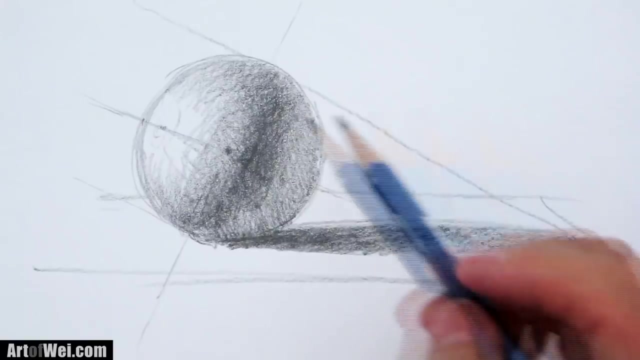 It seems like it's getting way too much light from the environment. I'm just going to darken it up a little bit and make this part darker. Okay, so let's see how that looks. That's kind of getting there, right. 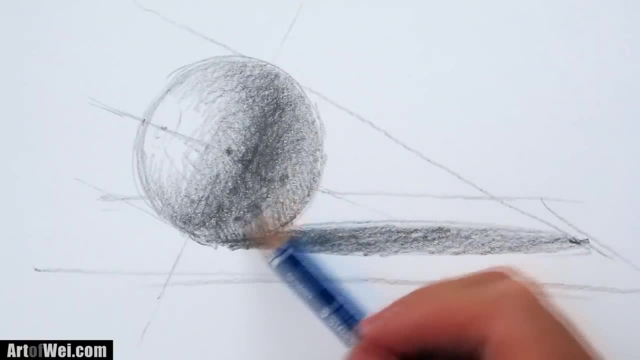 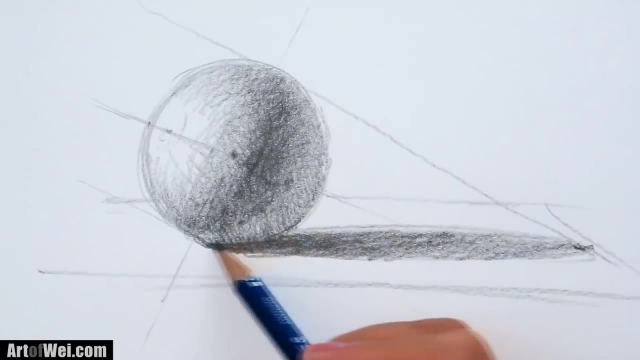 And usually with- and I'll go into a little bit more detail now- how to make this thing a little bit more realistic, because, you know, if we play with the shading a little bit, we can get them Much better form. 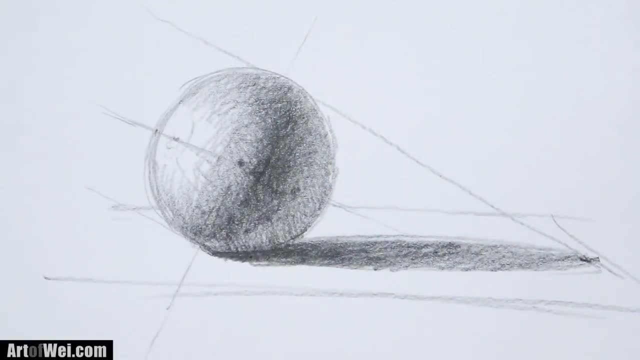 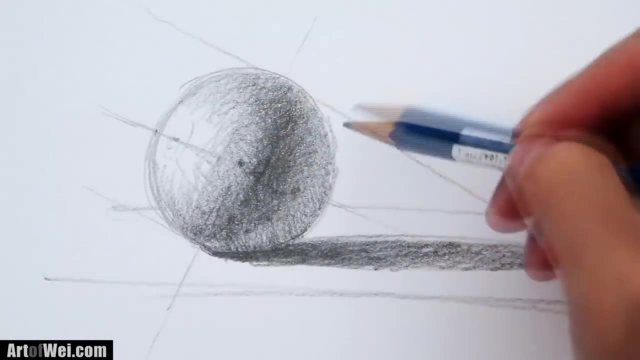 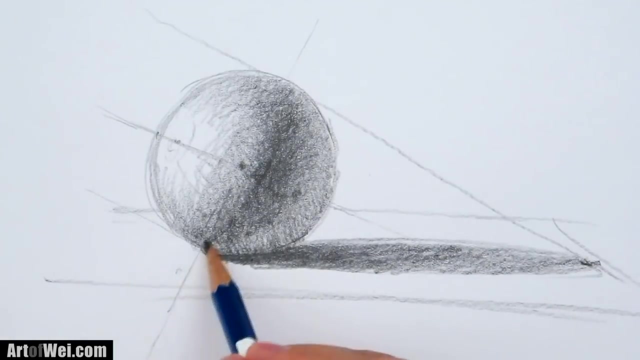 All right. so now we have this, which is pretty good, but with circles again, the environment is always, you know, hitting the edges of the sphere. So especially down here, you know this light source, right here, it's going to bounce back. 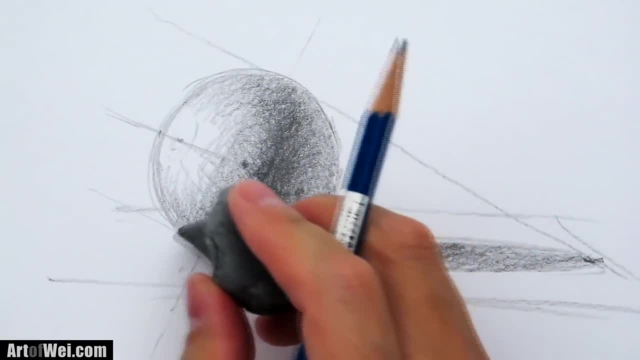 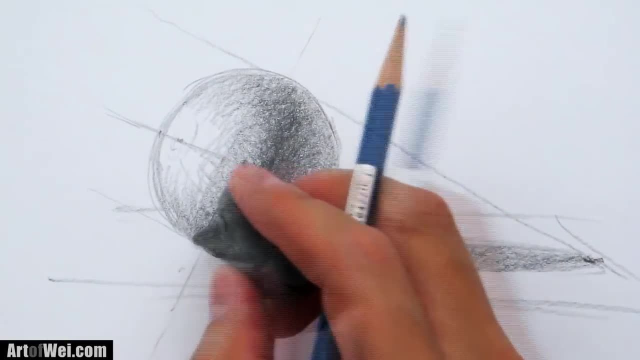 up here. I'm going to line up the circle right here, So I'm just going to dab it with my kneaded eraser and this will take away some of the shading. Okay, All right. So you see, now, by taking it out, you can see, you can feel it a little bit more, right? 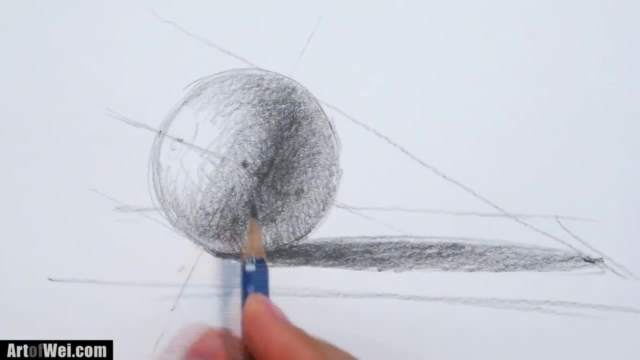 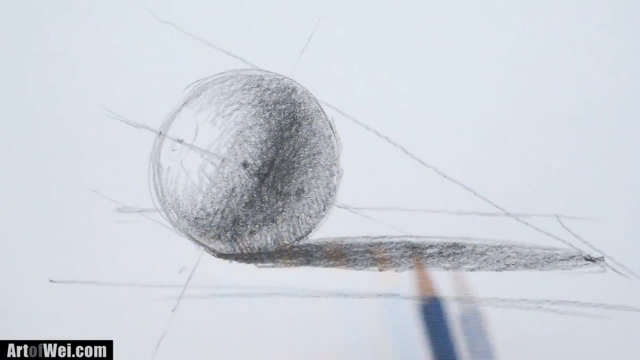 You feel like this is full of shape, So with circles, with spheres, it's actually very important to have this kind of stuff. So I'm going to make this part a little bit darker, just to put contrast, you know, into that edge, so that you feel like you know this part is light and then this part's darker. 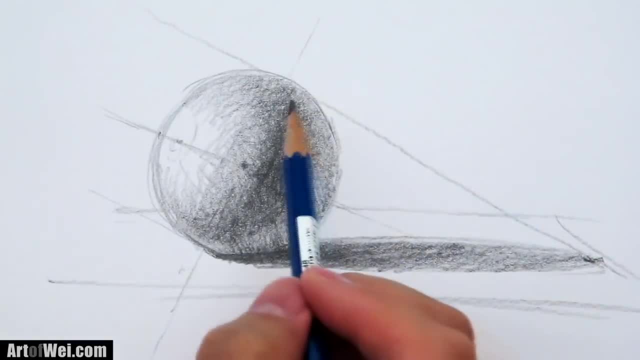 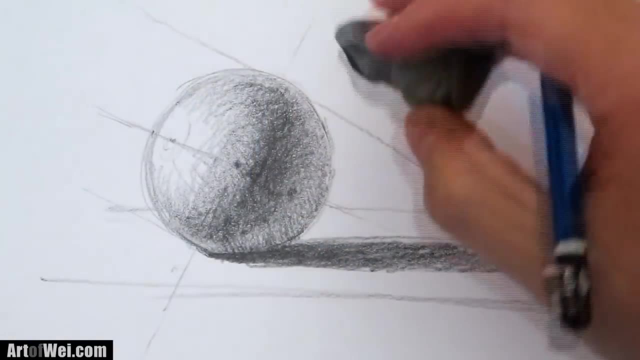 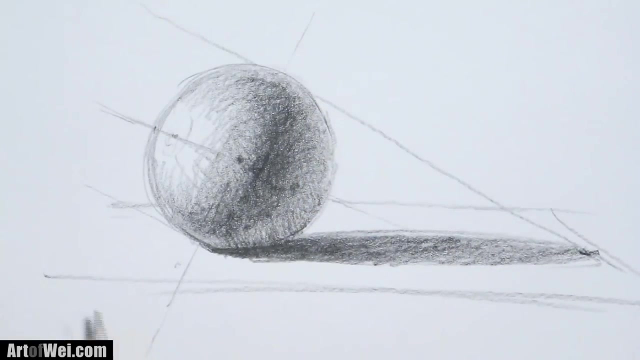 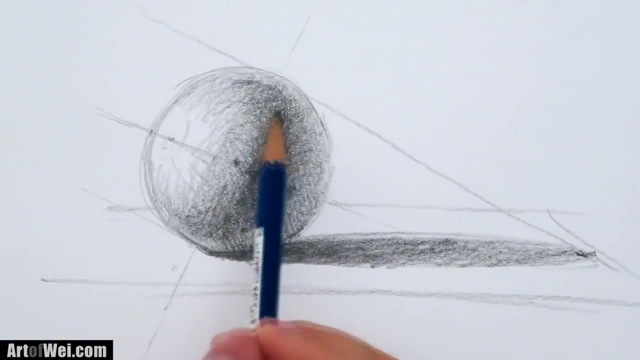 right. So, and in reality you know this whole area right here, this whole edge, So I'm just going to dab it because it's getting light from the environment, okay. So that's why when you see realistic, you know shading of a sphere, you have this kind. 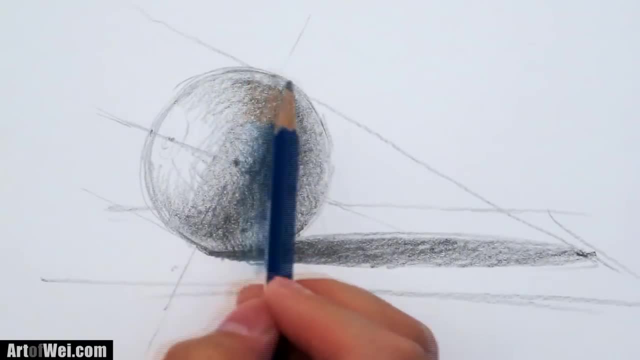 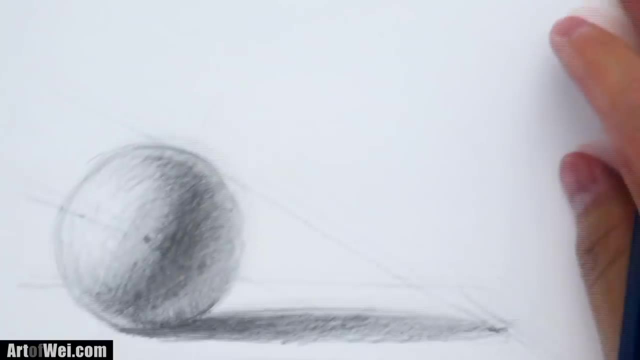 of shape like that, where the edge all around the edge is a little bit lighter. okay, Okay, All right. So it's kind of like, let's see, you can actually do it fairly quickly. It's kind of like a chrome sphere, right. 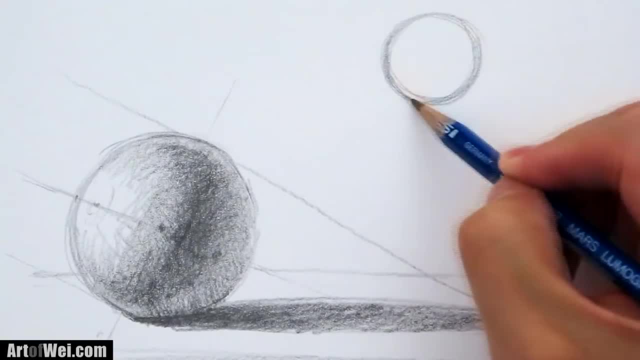 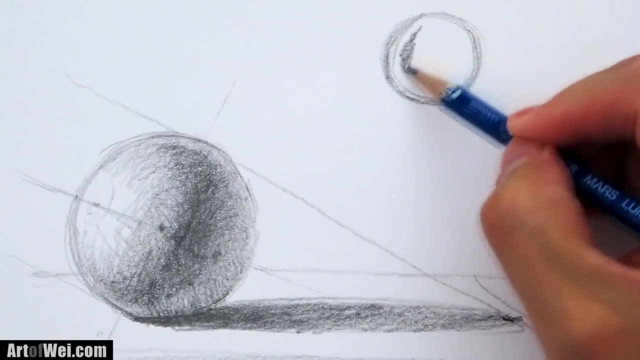 It was chrome. You know the edge, how the edge is practically all white because it's reflecting light and you can just shade it like this and you'll see. you can see a lot of this stuff. So you know, you just take a circle and you shade it like this. all of a sudden it 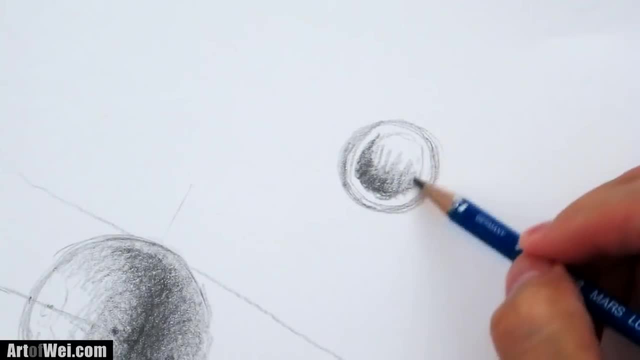 feels like a sphere, Right. Okay, So that's what's happening here. You know, it's just reflective light hitting back the edge, So we can shade this. See, like this part right here. it's pretty dark, right. 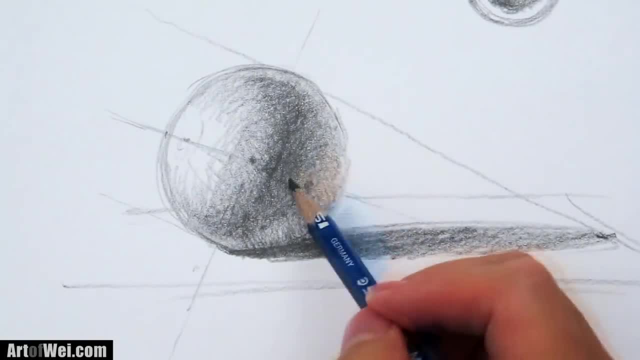 Right in the shadow area. So this area right here won't get a lot of reflective light, So this can be darker, Just right there, a little bit darker, Okay. So now it feels like more and more Okay. 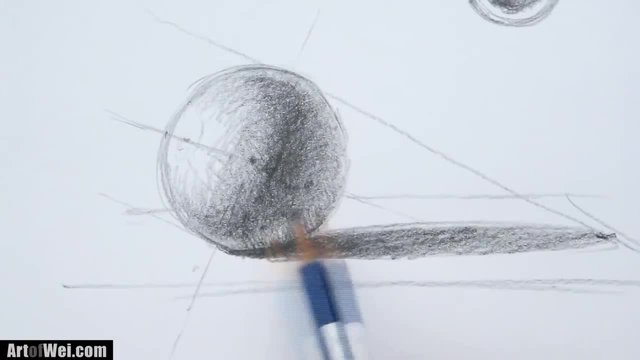 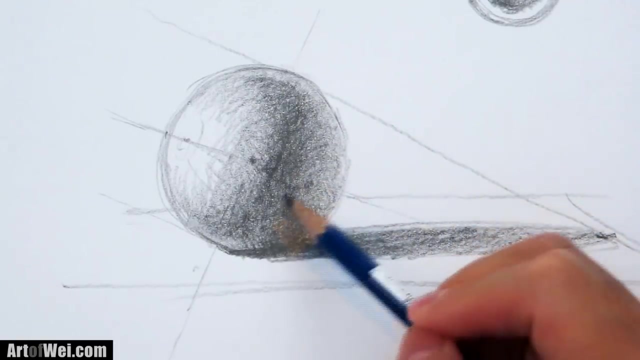 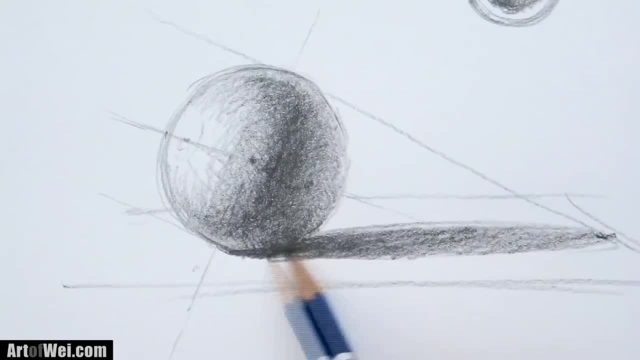 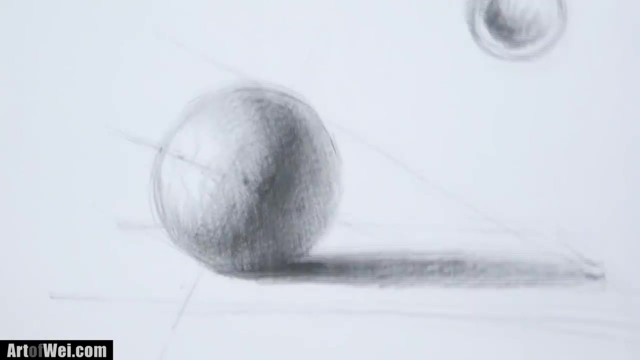 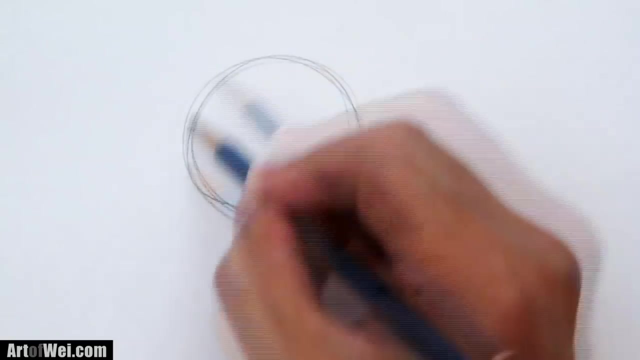